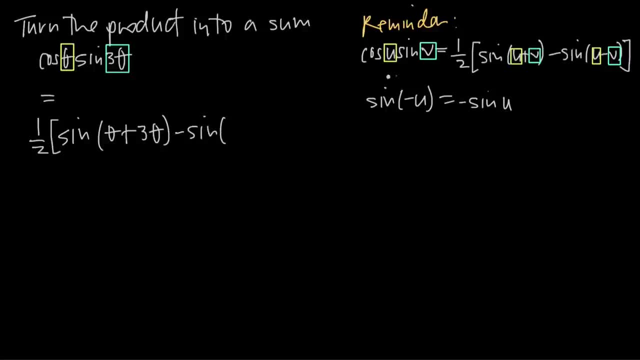 So minus sine of u minus v. Well, in that case, for us that's theta minus 3 theta, So that, and that's the end of our formula. So notice that this is already the difference of two sine functions. We just need to simplify it. 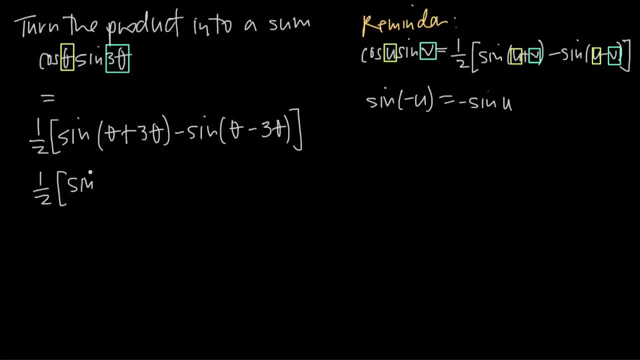 So we're going to get 1 half times sine theta plus 3 theta is 4 theta. So I'm going to get sine of 4 theta. and then here, minus sine theta, minus 3 theta is negative 2 theta. So I'm going to get 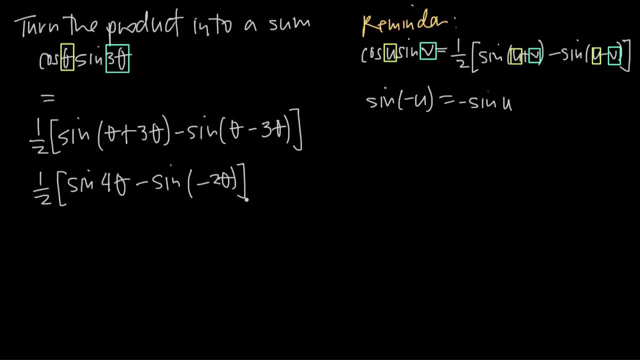 negative 2 theta. Now, technically I could leave the answer in this form, but it's a little messy having this negative angle. So in order to fix that, I can bring in this extra formula which tells me that sine of negative u is equal to negative sine of u. So when I have a negative angle, 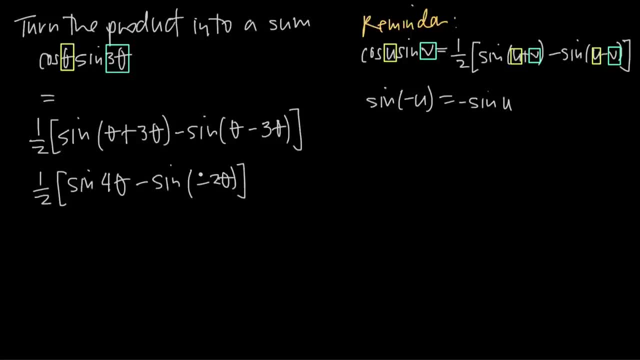 on a sine function. I can just pull that negative sign out in front. So I can take this negative sign, bring it out in front of the sine function and the negative times. the negative is going to be a positive. So I'm going to be left with 1 half times sine. 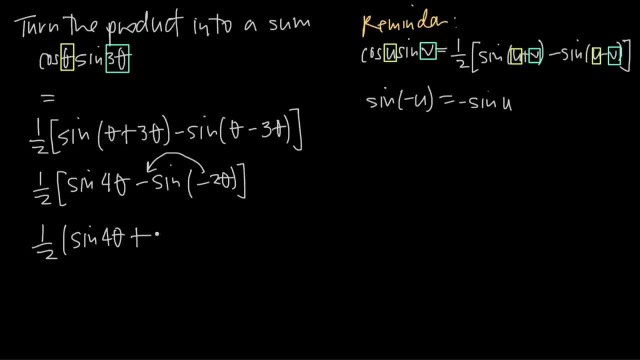 of 4 theta, and then instead of minus I'll have plus sine, and we brought that negative sign out in front. It made this a positive, so we're left with sine of 2 theta. I could leave my answer just like this. I could also go one more step. 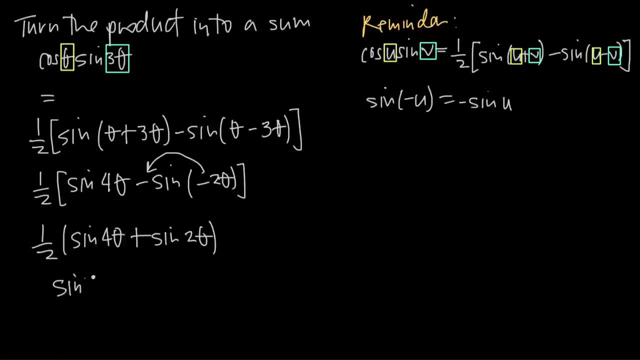 bringing the fraction into the two terms here and turning this into sine of 4 theta plus sine of 2 theta, all divided by 2.. Any of these answers are acceptable. This is probably the cleanest one, but in any of these cases, notice that we've turned what was a product into a sum. 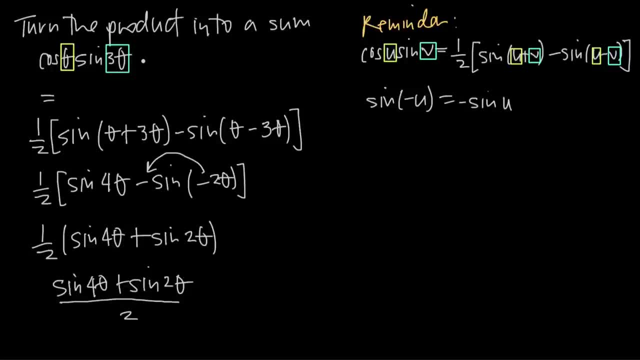 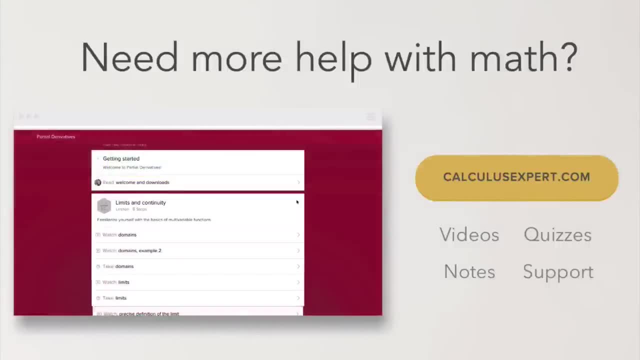 and that's how you use product-to-sum identities to manipulate a trigonometric function. Could you use some extra help with math? Click the button to head over to CalculusExpertcom. It's where I've collected and organized all of my best resources. 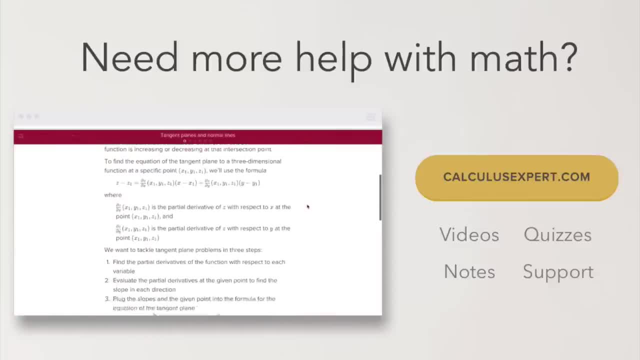 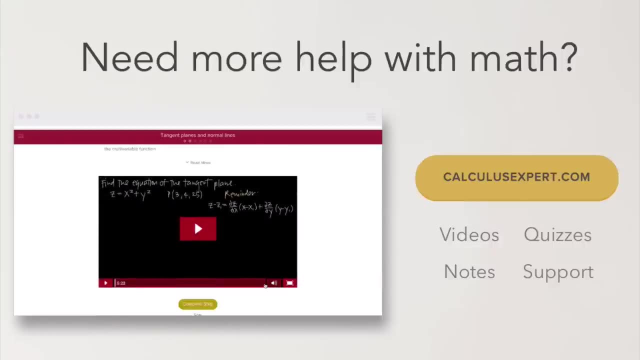 including exclusive videos, notes, quizzes and even formula sheets. It's the perfect resource, whether you're struggling, or if you want to take your learning further. or if you want to take your learning further, or even if you just want to save yourself some time studying. So check it out, because I know it'll help.